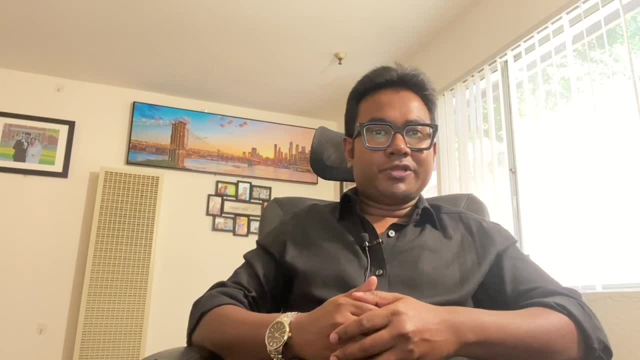 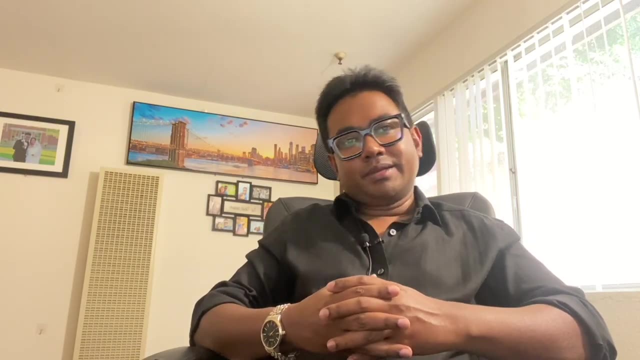 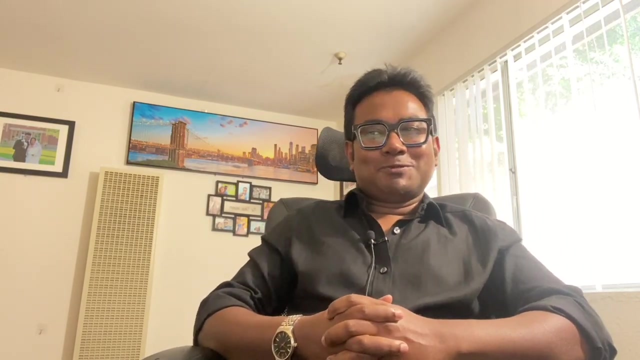 fifth part. i will give my very personal opinion, which i am uh, which i will mainly discuss- about what i feel. okay, it's not a it's not an expert opinion, but what is my opinion about it if you consider myself as an expert? okay, so let's go to the first section. 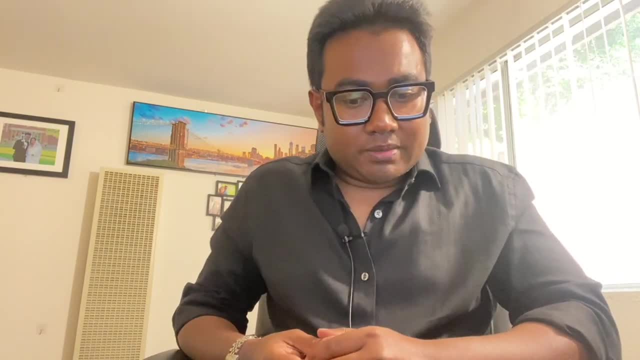 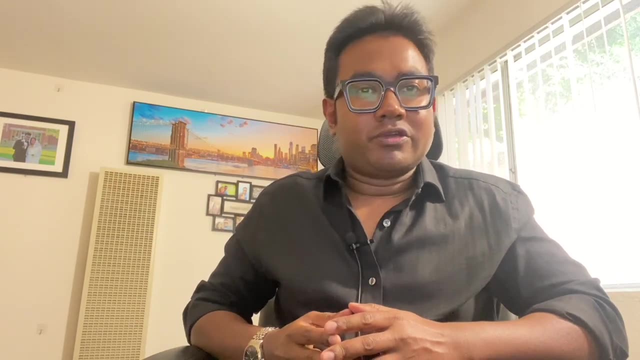 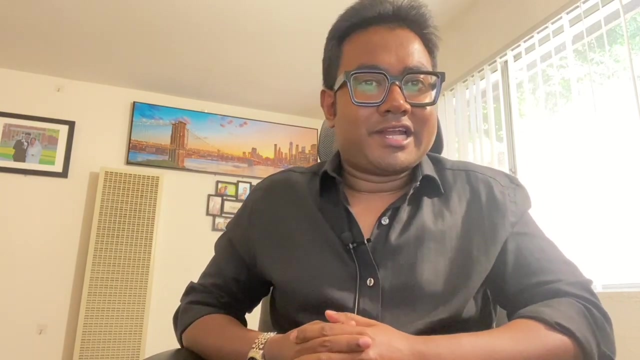 i will talk about study curriculum. so bachelor in aeronautical engineering program. this is mainly a four years long program. so if you take the aerospace or if you choose the avionics, they have their specific curriculum. when i studied aeronautical engineering at military institute, 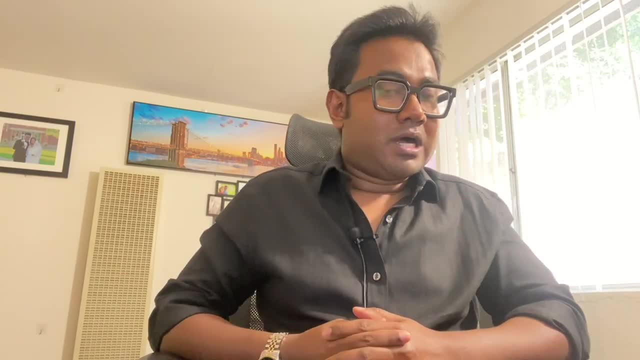 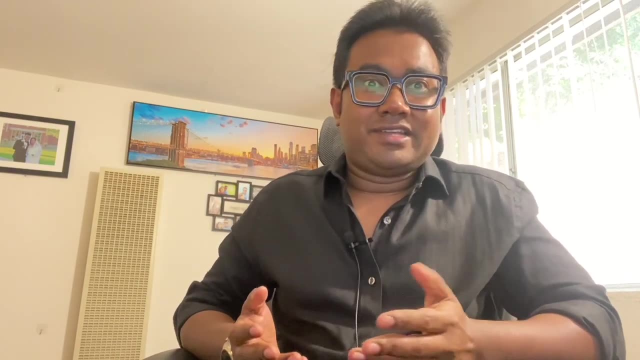 of science and technology, mist our aerospace and avionics. this separation was done when we were in the sophomore year or the second year or last year. i have completed my second year in avionics, echoes level two, but nowadays i'm listening that this separation is done at the very beginning. maybe. 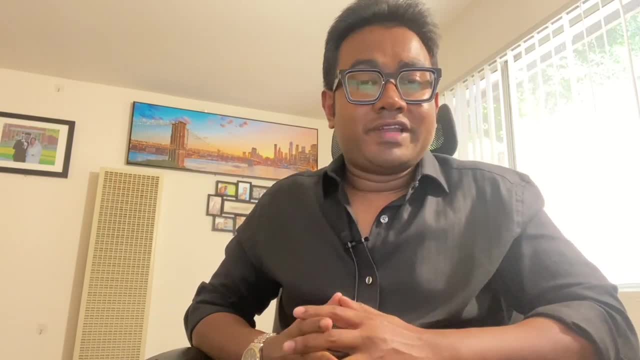 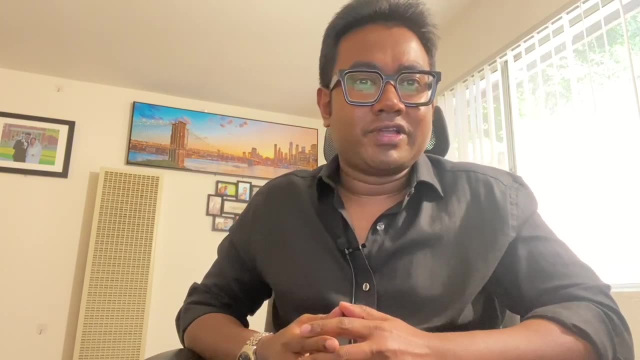 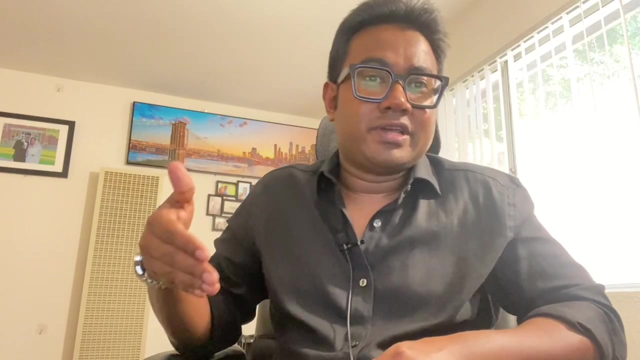 they have done some changes in the syllabus but whatever it is, for almost all the engineering program, not only aerospace or aeronautical or avionics, for all the engineering program first two years, like the junior year and the sophomore year- sorry, the freshman year and the sophomore. 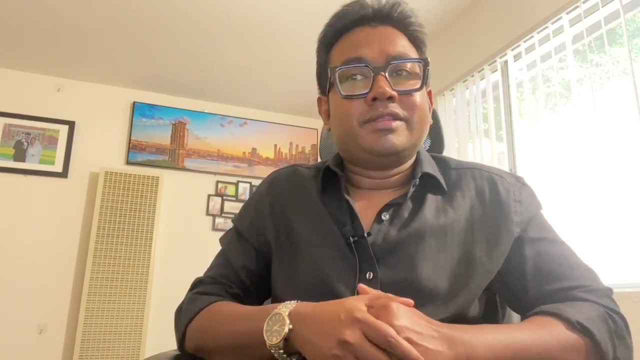 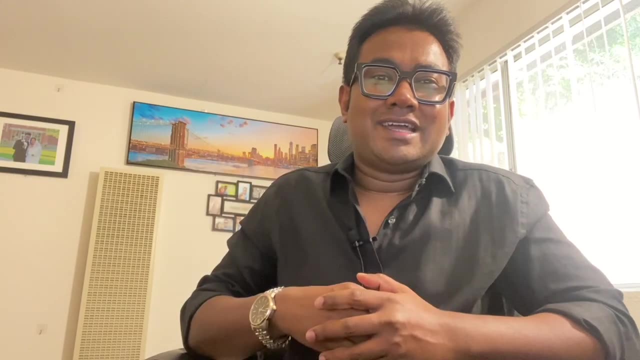 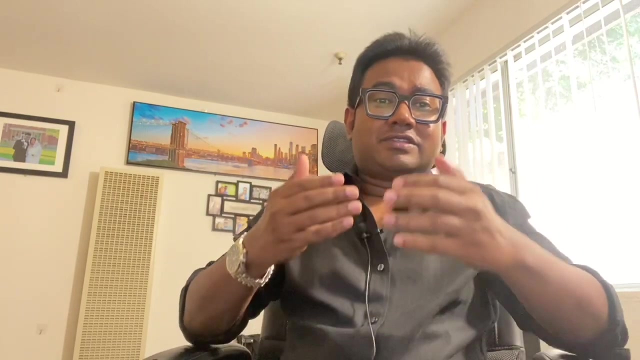 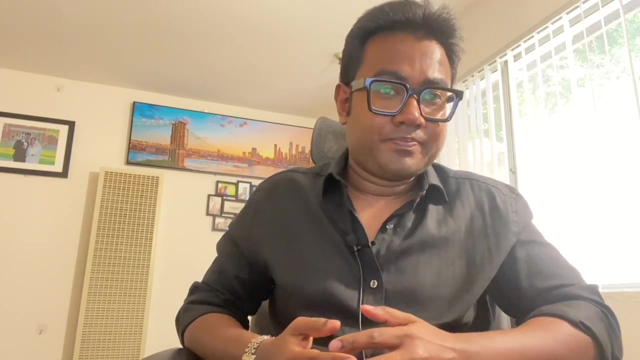 year. that means level one and level two. they have almost the same identical syllabus like, mainly focused on mathematics, physics, sociology and some other common discipline are taught or subject are taught during that time. so the main difference come from the junior year and the senior year. that means level three and level four, or third year and fourth year. here you will see. 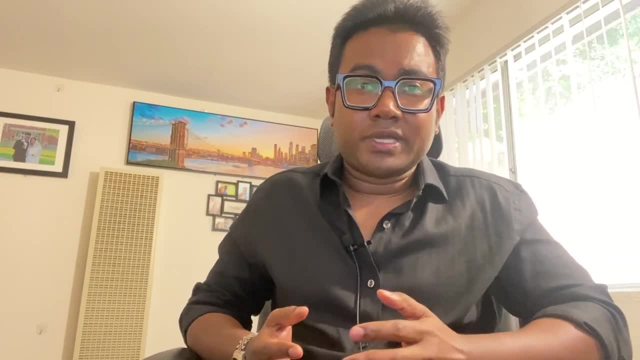 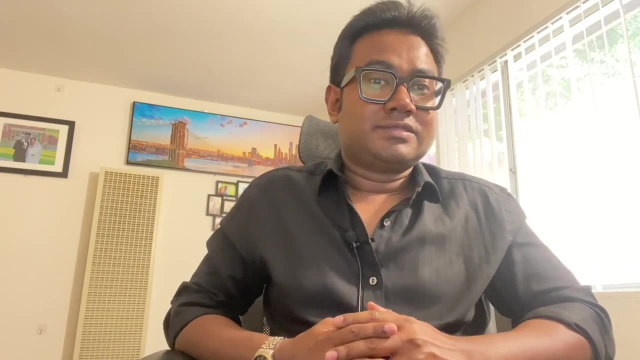 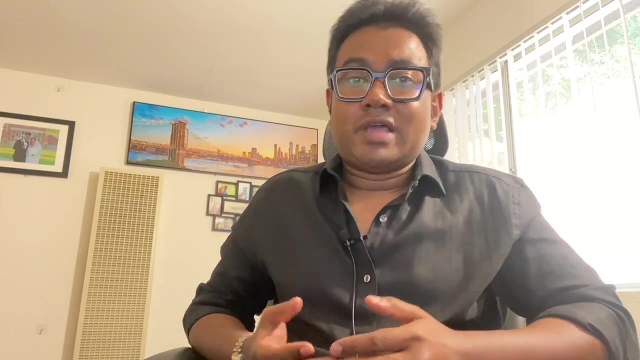 the significant differences. so i am assuming the syllabus for the first two years is same for the aerospace and the avionics. if i consider during my time when i started from the level three and level four, you will have a separation. we will have a different discipline, a different subject, like if you go for aerospace. 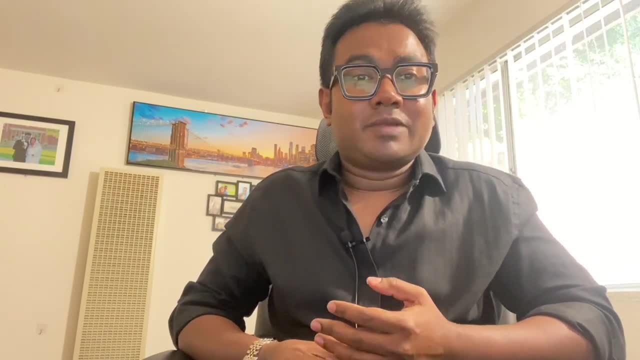 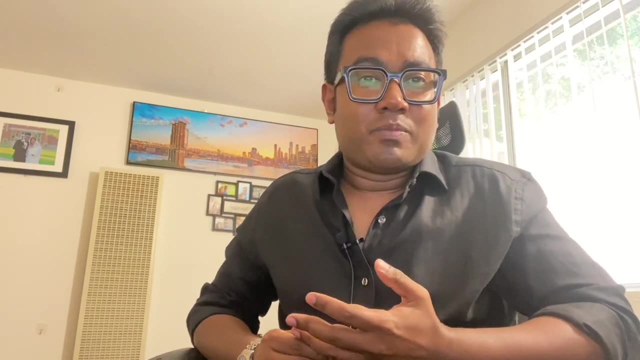 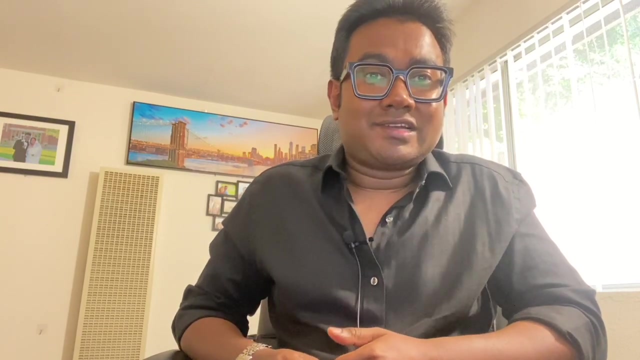 engineering, you will mainly focusing on the mechanical parts of the airplane. like your main study subject or focus will be aerodynamics: airplane design, aircraft performance, spacecraft propulsion or rocket propulsion, aerospace propulsion and also the structural analysis, aerospace structure. so this will be your main bread and butter and you will also study about the 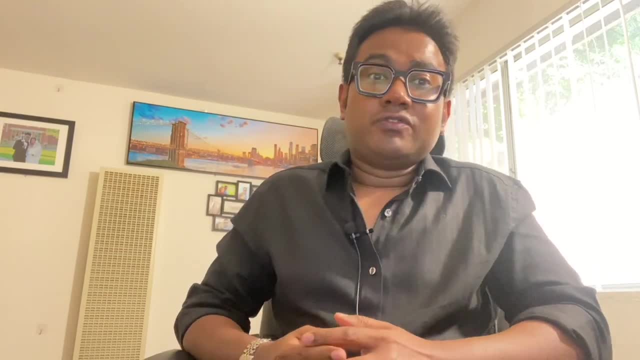 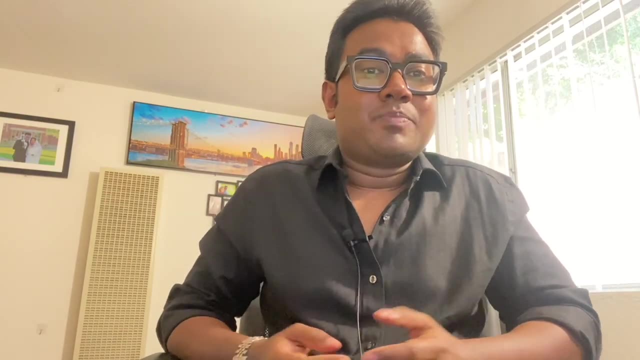 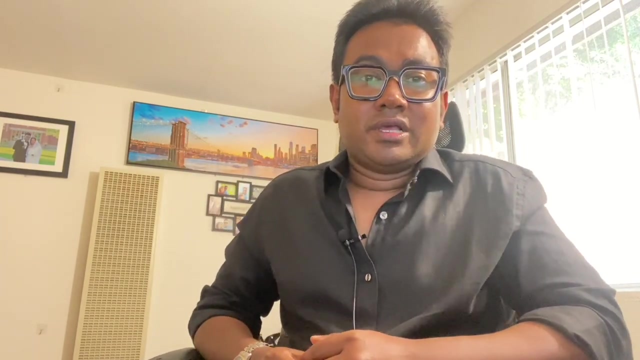 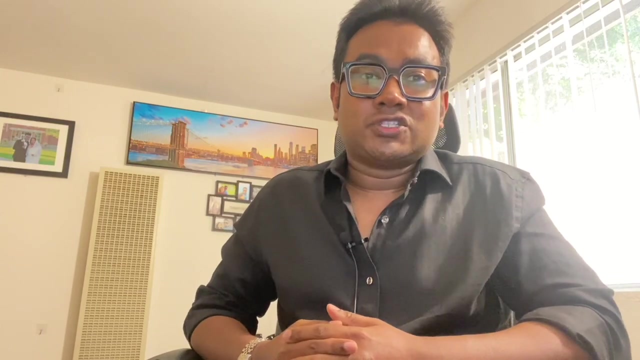 helicopter flight dynamics and other things. and if you choose the avionics, on the other hand, you will mainly focused on the navigational parts and the electrical part or electronics part of the airplane. you will study radar, radar engineering, radar navigation. you will study about different navigation system like vor and vhf, different communication sort. 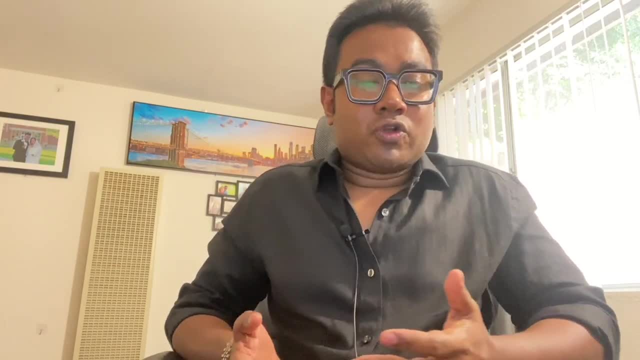 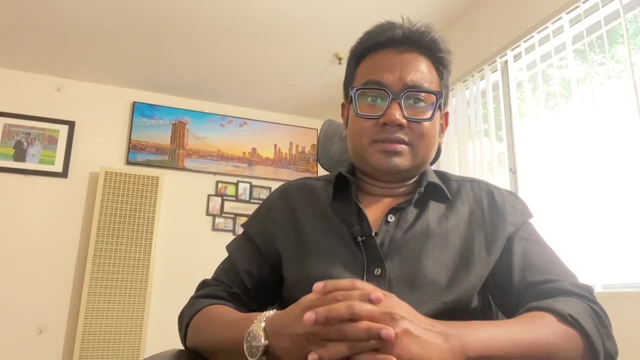 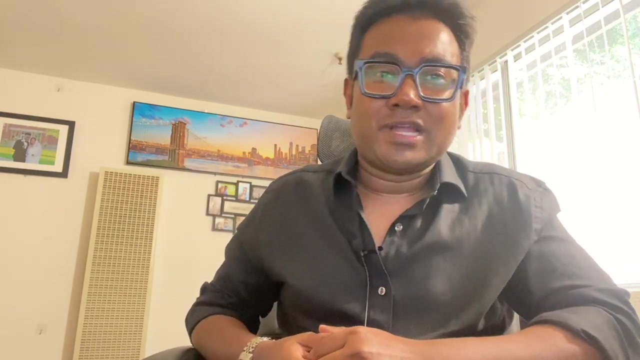 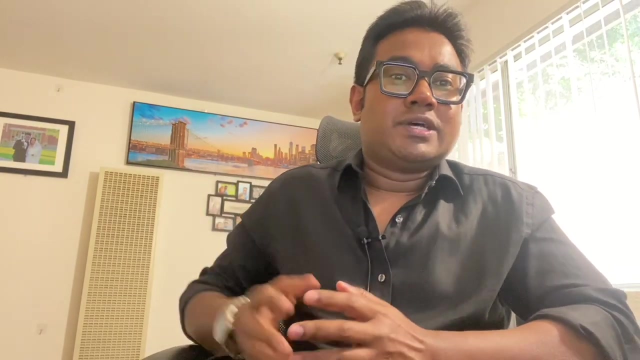 that uh airplane use a microcontroller and other common electrical engineering subject. this will be your main study topics. so this is about your study curriculum. if you are someone interested about mechanical sort of subjects like aerodynamics and others- propulsion, thermal side, material side that i said earlier- then you can easily choose the aerospace. and if you are someone, 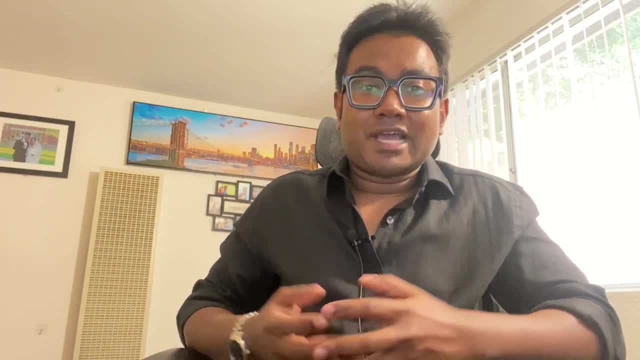 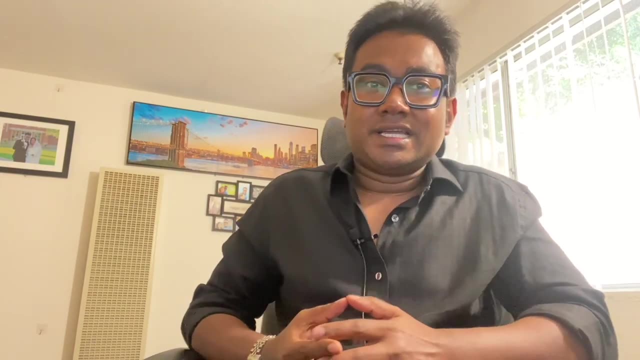 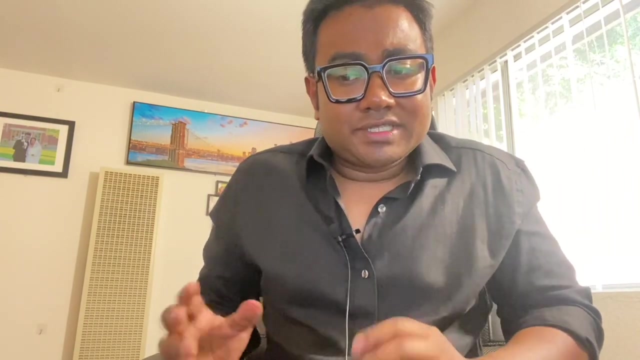 who is interested mostly about the electrical engineering types of subjects like microcontroller navigation, radar communications, communications engineering. in that case, you can easily choose the electric avionics side. okay, avionics track. so this is the main. uh, this is a synopsis of the curriculum that you are going to study. 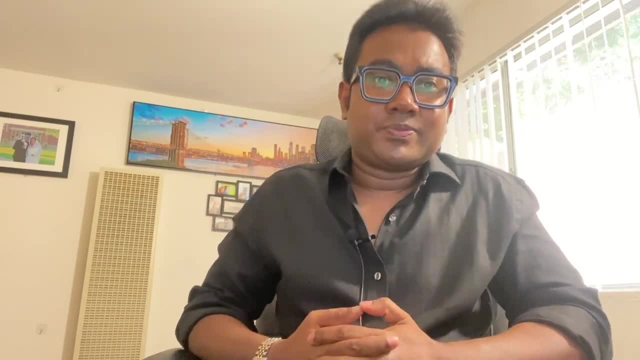 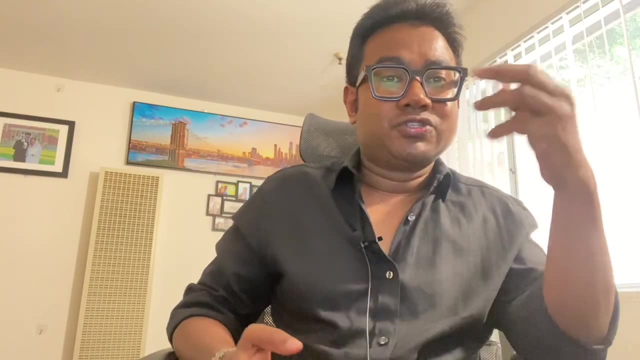 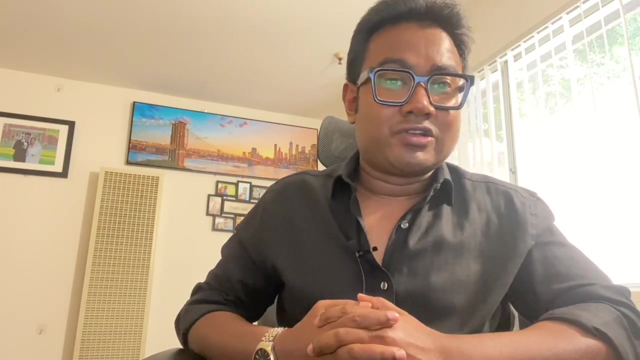 now we will go for the job sector, job sector in bangladesh. after graduating from mist, i took my job uh in novoyar at domestic airlines in bangladesh. so if i said with prospect to novoyar, both from aerospace and avionics, people are recruited during our time as a trainee engineer. 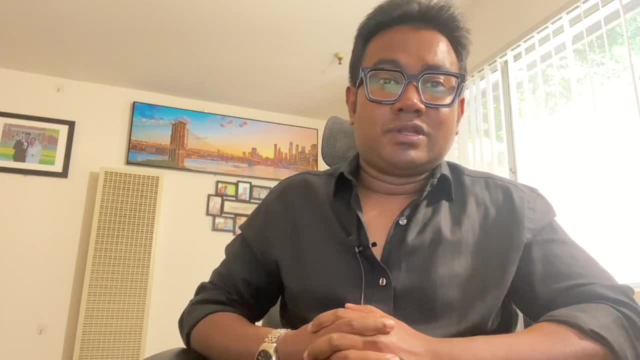 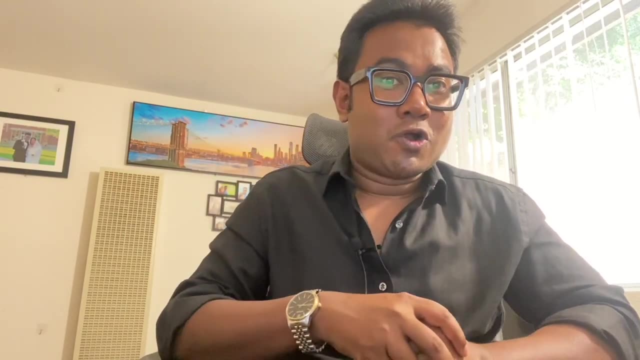 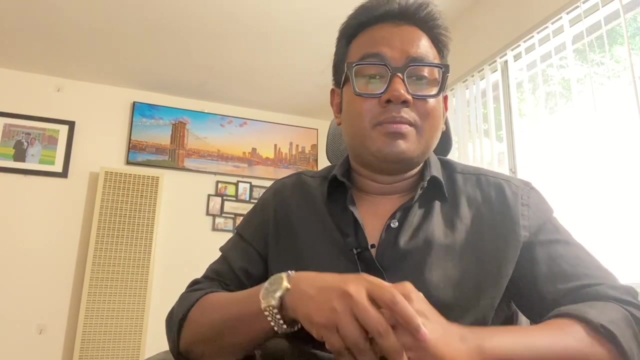 so, if you ask me, yes, the opportunity is equal, no matter if you study aerospace or avionics, but there are some extra advantages that the avionics people got during my time, what i want to mention here: during my time, when i studied a mist, we have a more number of students actually studied aerospace than the avionics. 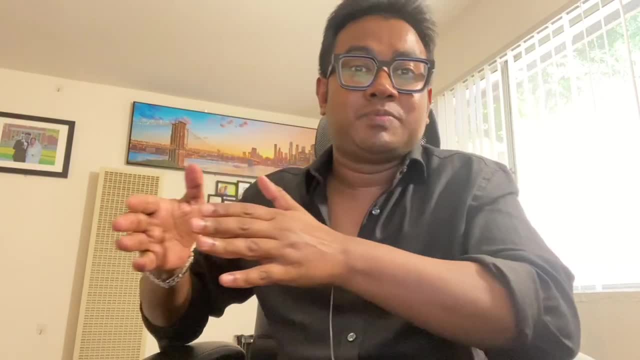 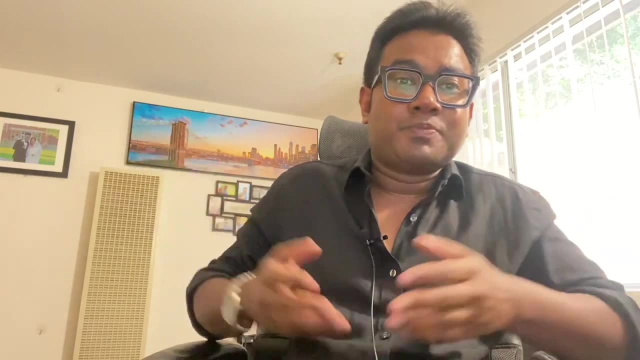 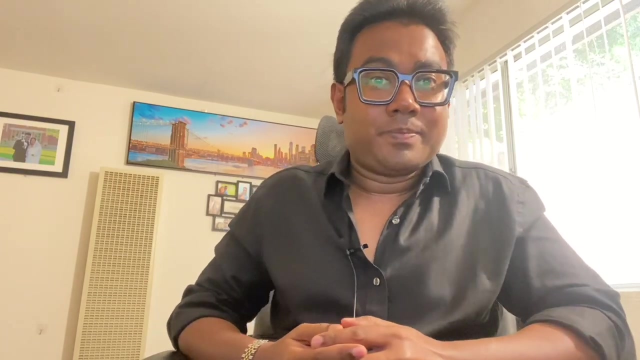 and maybe their number was half of the people who studied aerospace. so if we have fifth uh 20 students for the aerospace, we have 10 students for avionics. so that's a just simple example for you. so when we went to the airlines and when the airlines offered us the type training program, 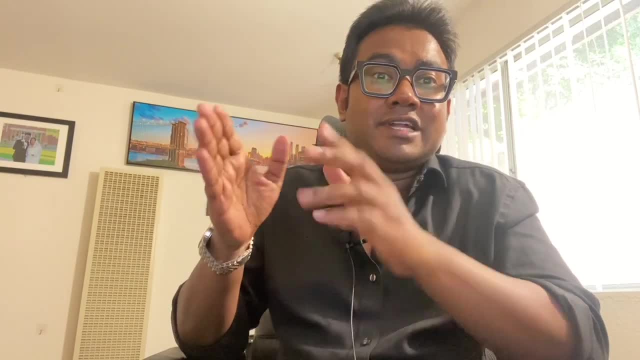 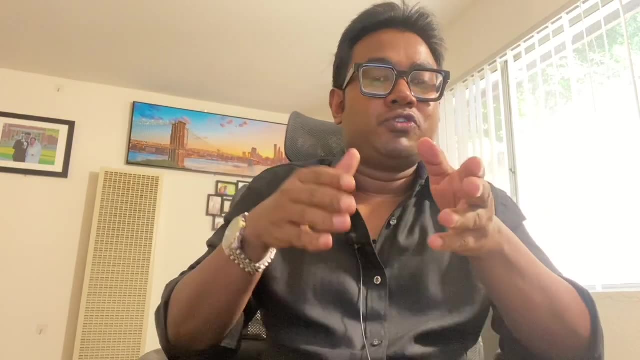 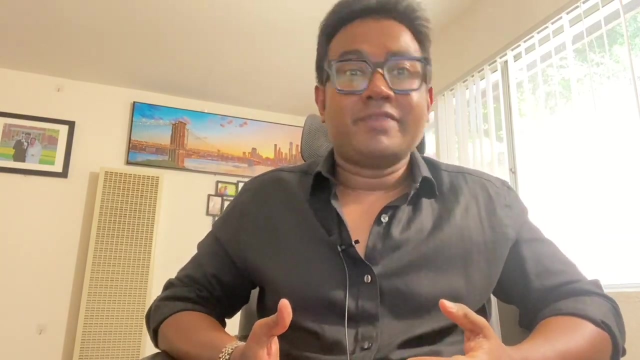 so we found that we have more people from aerospace, that is, b1, than the people from avionics, which are b2. this is their language in the airlines: b1 and b2: b1 is aerospace, b2 is avionics. so type training is a very desired thing for the engineers who are recruited to the airlines. everyone wants to. 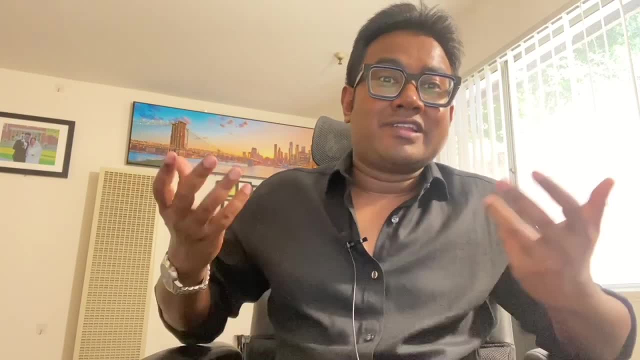 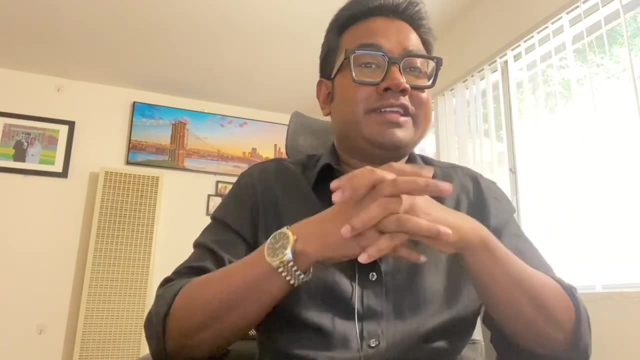 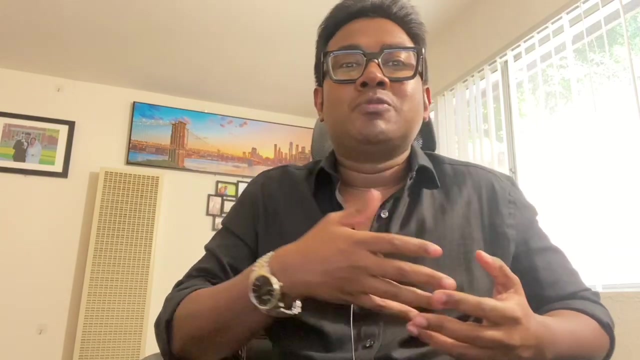 do the type training because it is related to salary incrementer the other thing. so during that time i found that between among the aerospace people the competition is very intense. not everyone was selected for the type training but for avionics, because the competition was less during our time. so the almost all the avionics people had 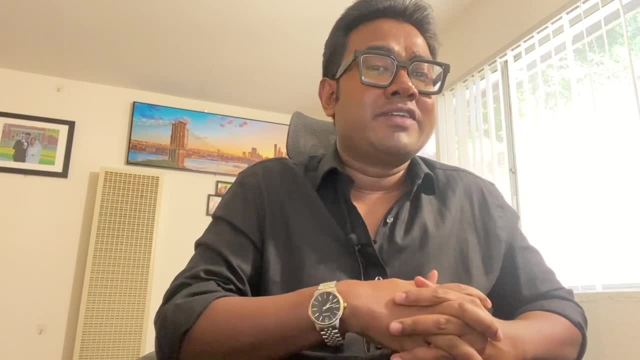 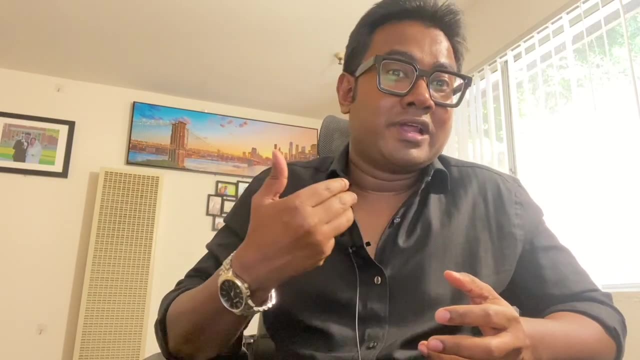 opportunity to do the type training. so this is a big advantage of avionics in Bangladesh job sector. I don't know the current situation. I am outside. I am abroad and living in the United States for the last five years, so things might change during this time. so always talk with the 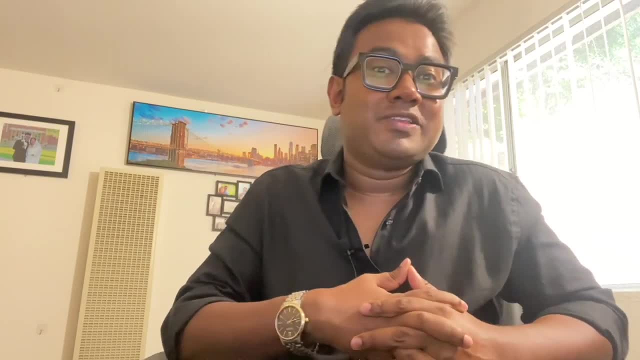 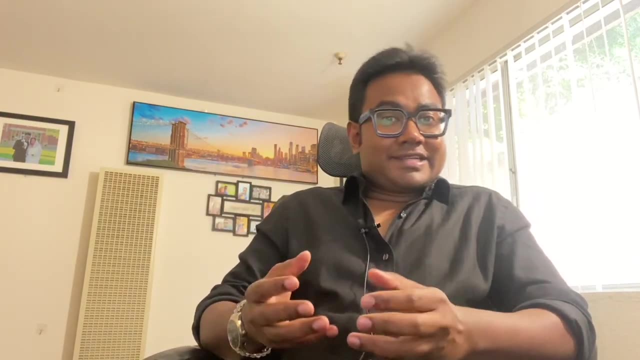 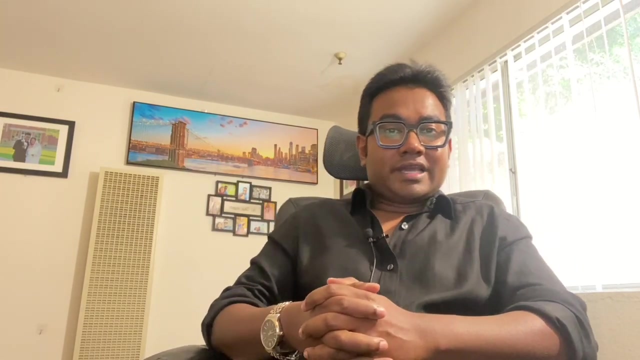 people, or contemporary people who are working at that time in the airlines. okay, now going for the higher study, and that is the third part for higher study, also similar to the jobs in Bangladesh. I believe there are equal opportunity both for aerospace and for the avionics. like you studied aeronautical engineering and your track was aerospace, for example, 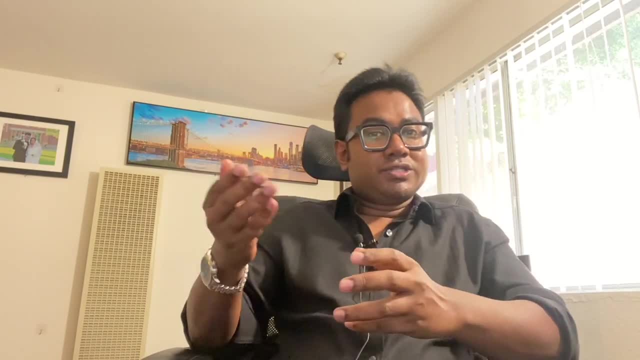 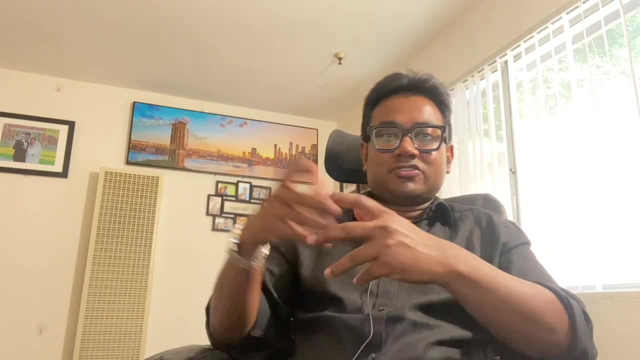 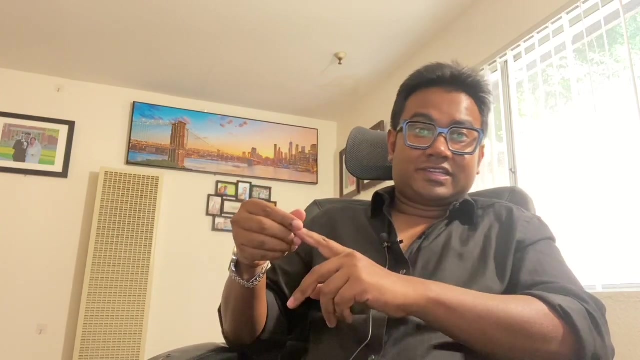 now you do not want to stay in aerospace field, you want to switch. you can easily go for mechanical engineering, material science and engineering, structural engineering, fluid dynamics or any other field. okay. similarly, if you studied aeronautical engineering by tracking that, by taking the track of avionics, engineering, still now, 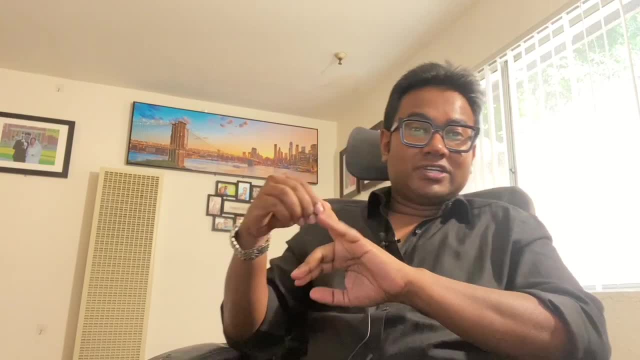 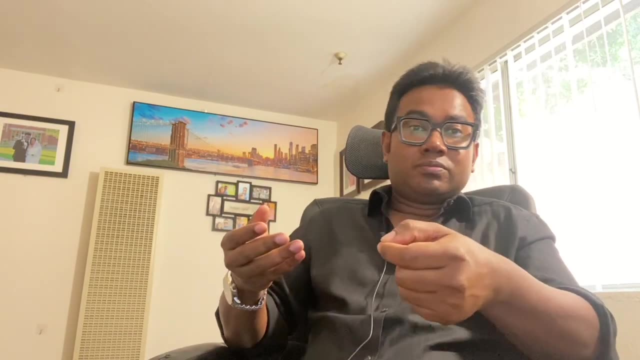 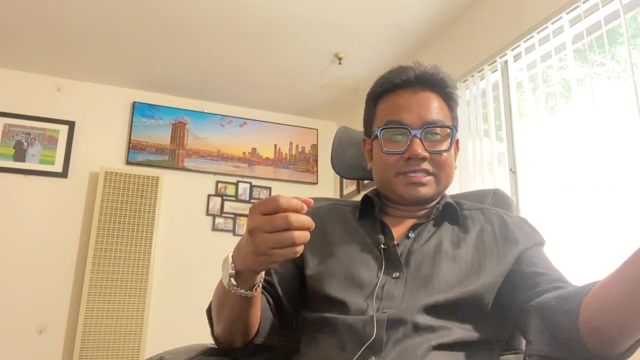 you have the opportunity to go for electrical engineering, computer science- okay, you can choose from these majors as well. beside your avionics, core major, beside your avionics- or aerospace majors- okay, you can always study aerospace engineering, you always study avionics. but if you want to change, 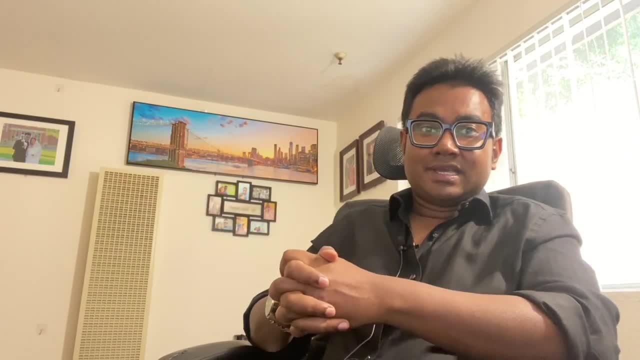 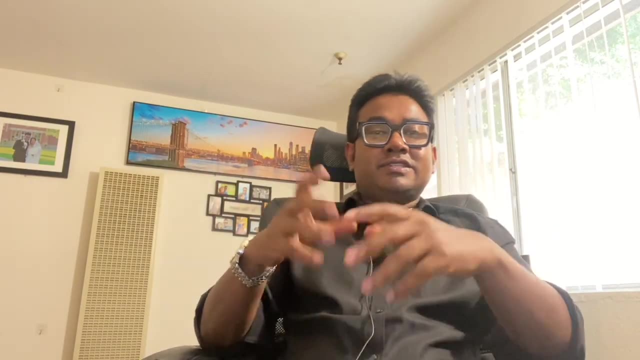 this is. there is option still now for you for your masters and PhD, and I always recommend people, or suggest people if you have interest. if you studied aerospace, you can always choose mechanical. it will give you the opportunity of your profile and improve your chances of getting employed in the 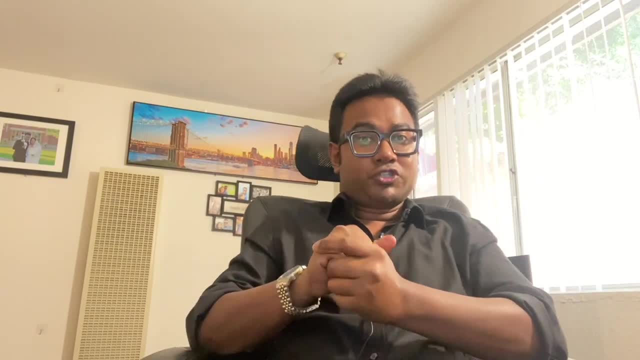 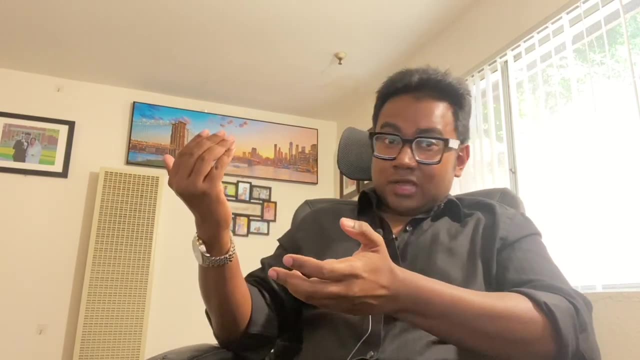 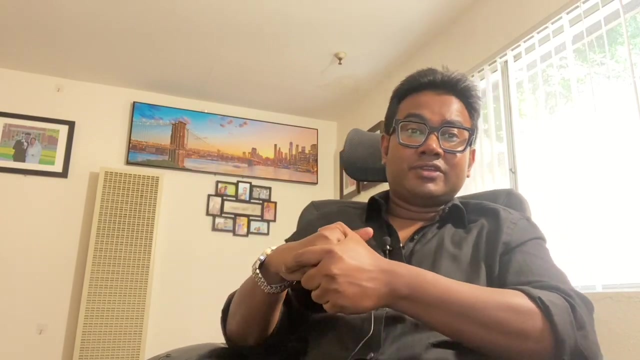 United States or any other countries that you are planning to visit. okay, that's a good, good choice. so higher state opportunities, also same. and the job in abroad, like I want to talk about job in the United States, for example, you studied aerospace in Bangladesh. now you studied mechanical in the. 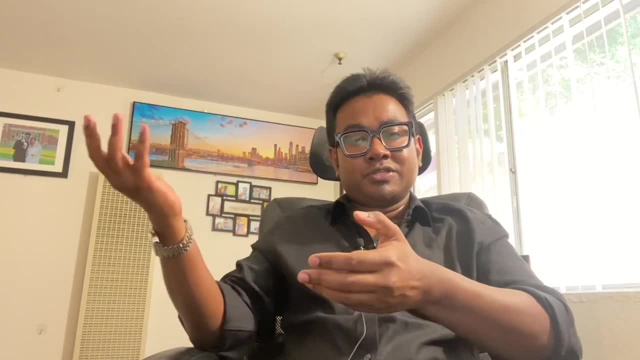 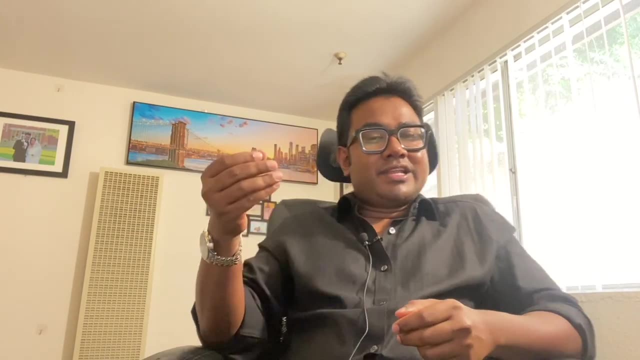 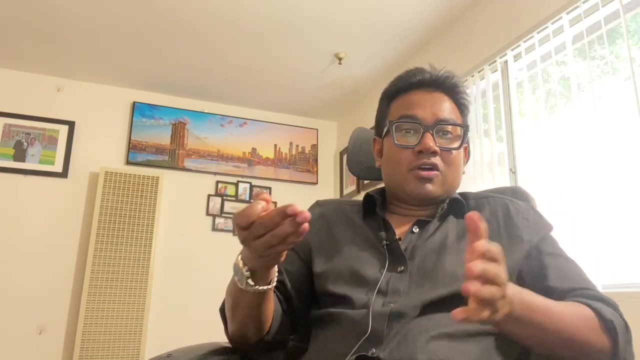 United States. so or you studied aerospace- yeah, your job, job opportunities available here. similar thing if you study avionics in Bangladesh and you choose electrical engineering, or you still pursue your aerospace engineering degree, masters or PhD, in the United States, but your major was, or focused on it was. 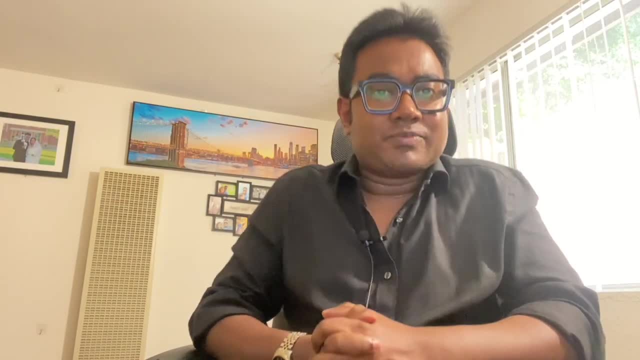 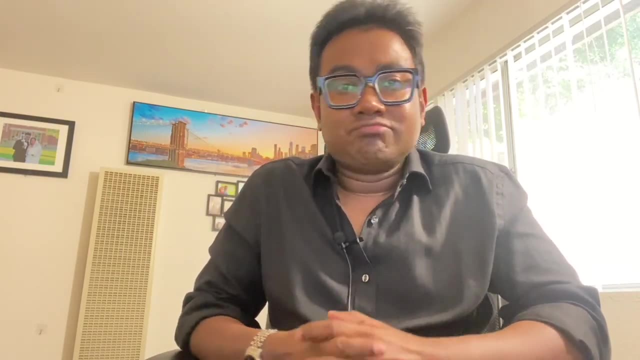 avionics focus like radar engineering, communication engineering, some sort of this. still now, there is a plenty of job for you in the aviation industry to work as an avionics engineer. so in terms of job, I believe there is no discrimination. maybe there are slight difference in the number of 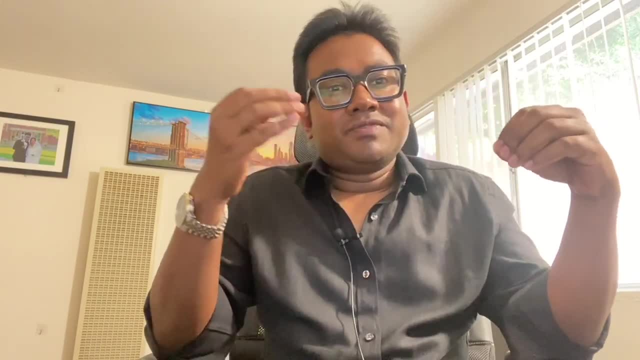 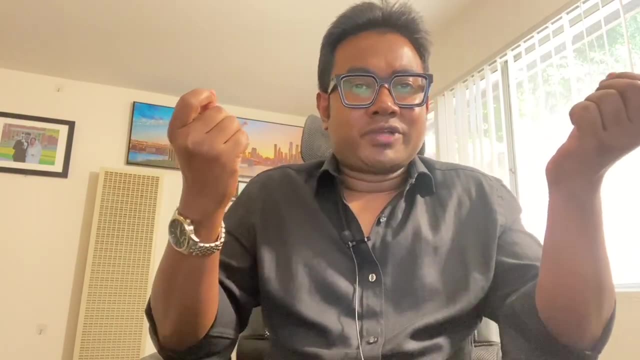 position available. sometimes there is more opening for aerospace and sometimes there is more opening for avionics, but there is still now pretty much same. so you cannot make a solid comparison between them. so I would want I want to say that for jobs in abroad, almost both are equal. 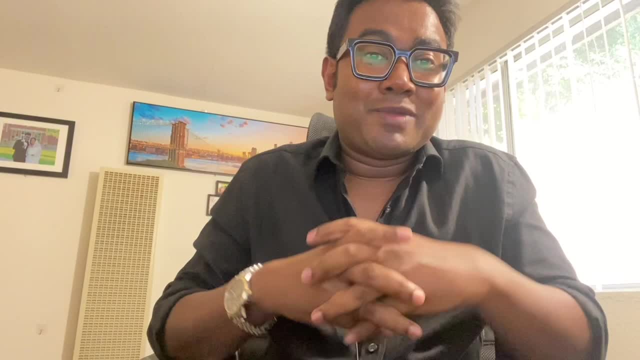 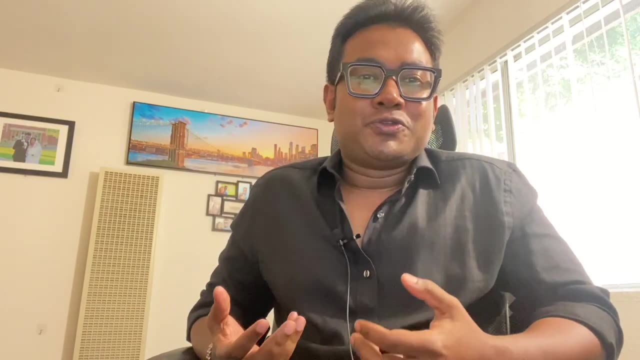 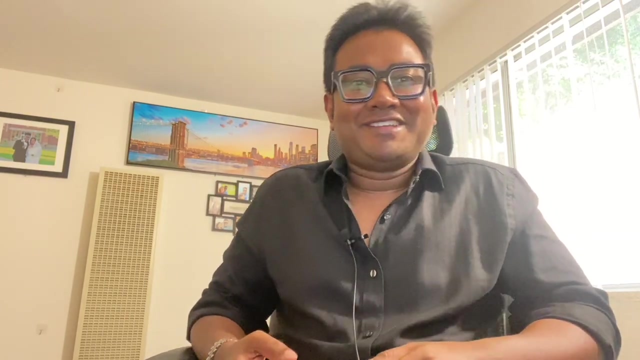 so fourth part is done. now the fifth part, which is my own opinion, if you consider myself as an expert, so just take my opinion. you don't need to take it very seriously. you can always consult with others, but if you want to take it, you can take it, because I studied aeronautical engineering. 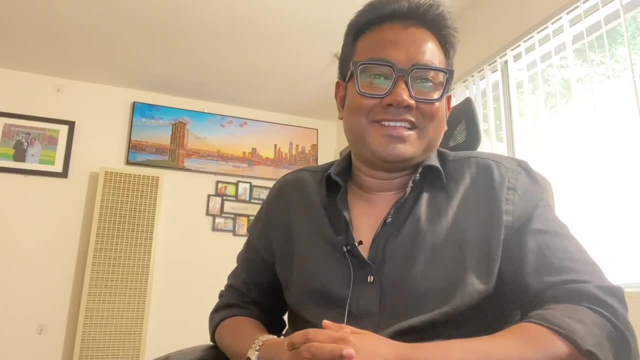 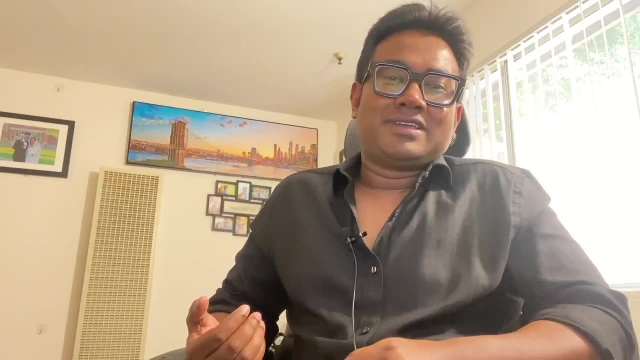 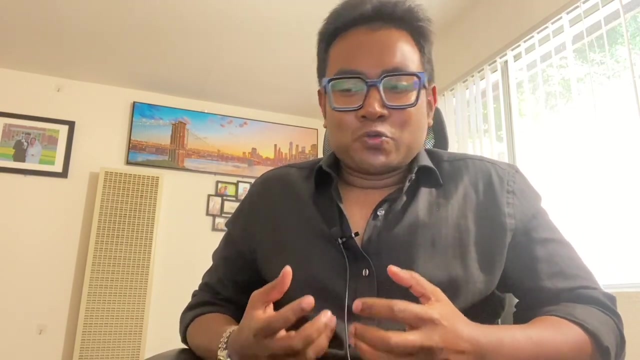 in Bangladesh. then, after my graduation, I worked in Novo air as an engineer. after that I came to the United States to pursue my higher study, completed my masters from here, now working at Boeing as an aerospace engineer. so with this experience, I want to share that why we study aerospace engineering, or why we study aeronautical engineering in Bangladesh. 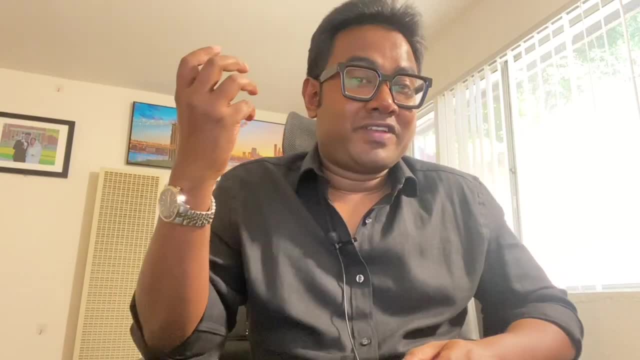 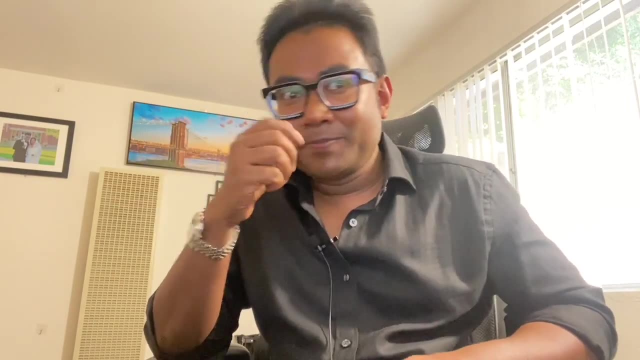 leaving all other majors, like during my time I saw we have some friends and seniors who got chance at Buet but even though leaving Buet, they came to my institute to study aeronautical engineering. why? the answer is very simple: they love airplane, they have obsession for airplane. okay, 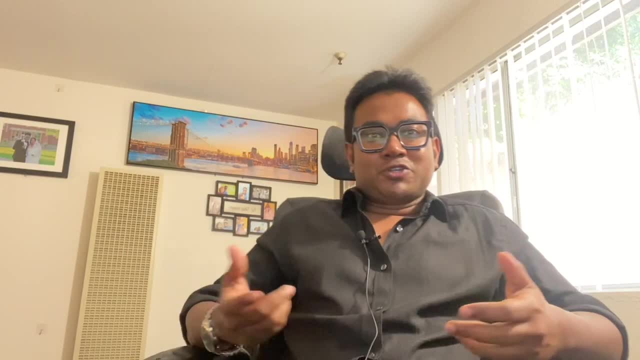 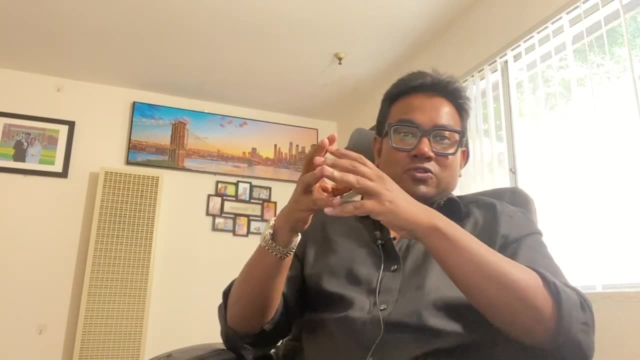 and when we say an aerospace engineer, both in USA, in Bangladesh or in any other country, we understand the people who design the airplane. okay, who design the airplane in Boeing also, there are a lot of job. maybe there are hundreds types, hundreds of jobs in engineering or aerospace. 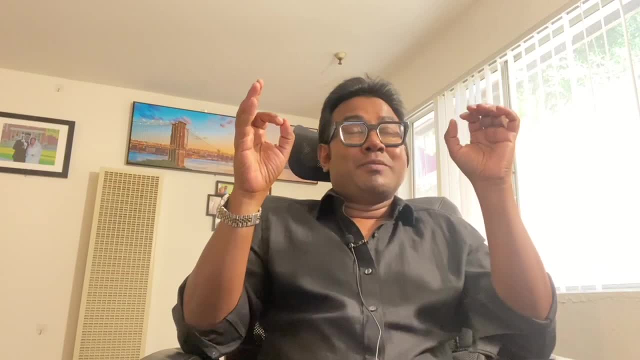 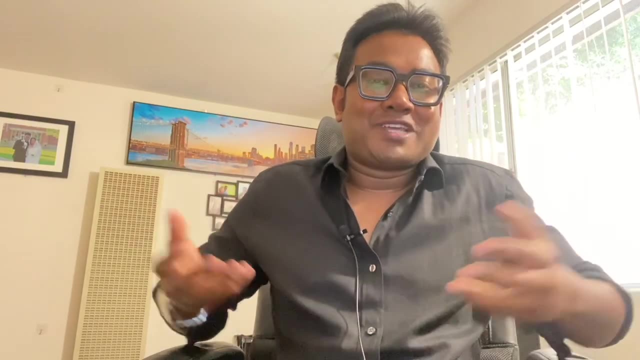 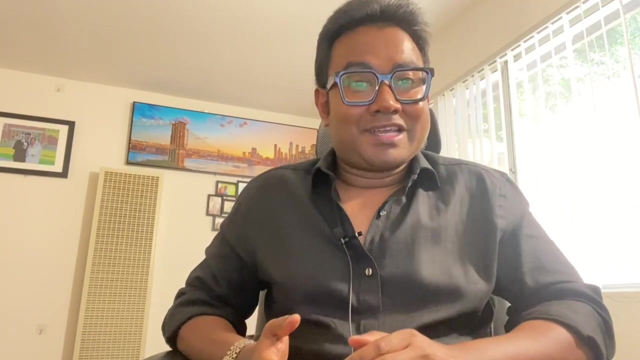 engineering. but do you know what are the main people? who are the main people in this field? the people who design the airplane. they are the top people in this field. okay, everyone wants to become an airplane design engineer who study aerospace engineering or aeronautical engineering, and you can only become an airplane design engineer if you study aeronautical engineering. 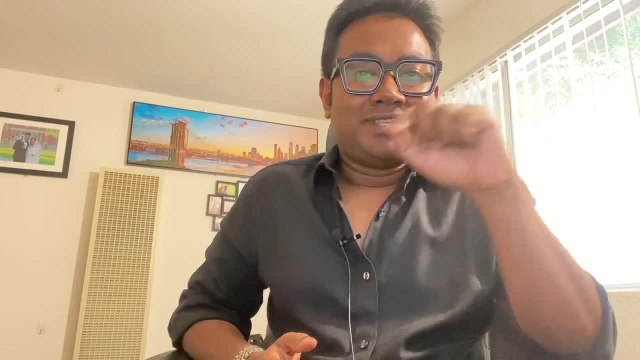 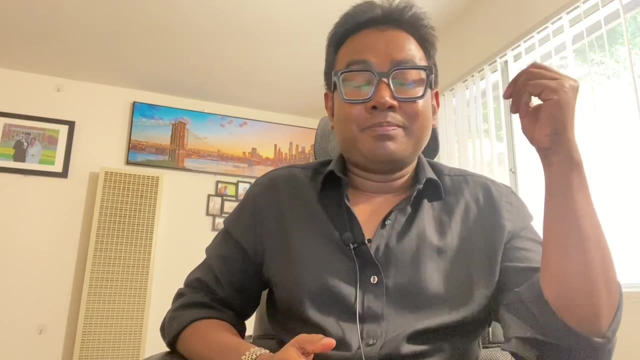 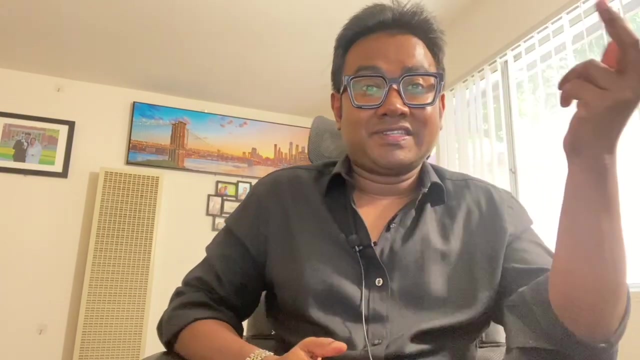 and if you study aerospace track, okay, because in this aerospace track you will be taught airplane design or aircraft design, or the course name can be aerospace vehicle design. you will be studied aircraft performance. you will be studied high speed aerodynamics, basic aerodynamics or fundamental aerodynamics. so these are the course which will make you an airplane design engineer. okay. 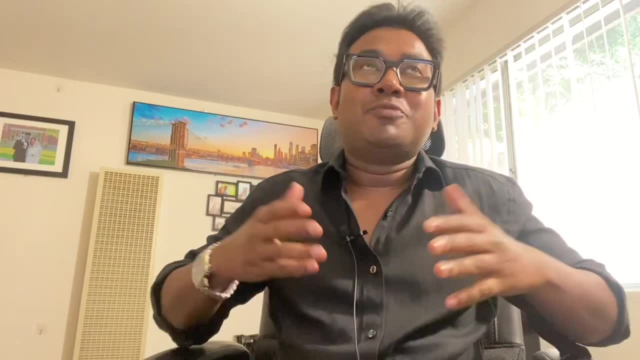 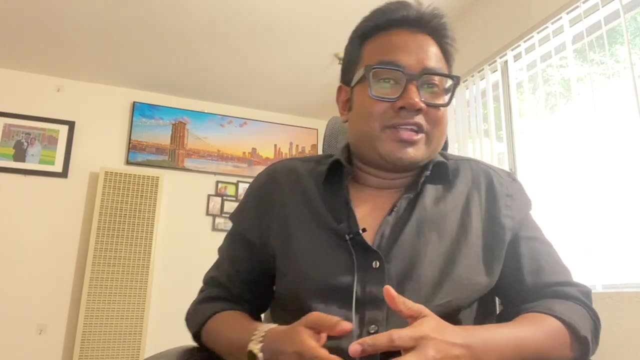 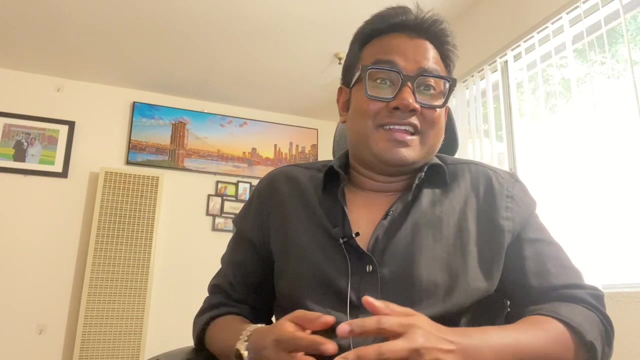 if you study avionics, unfortunately you you cannot become an airplane design engineer, so this is pretty much common. you can become a navigation, navigation and control engineer, you can become a radio communication engineer, you can become a satellite design engineer, but you cannot become an airplane design engineer. 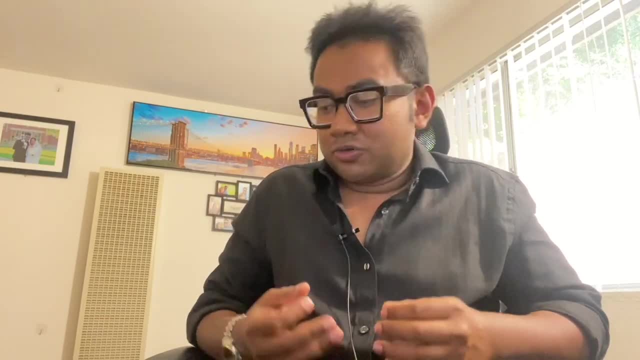 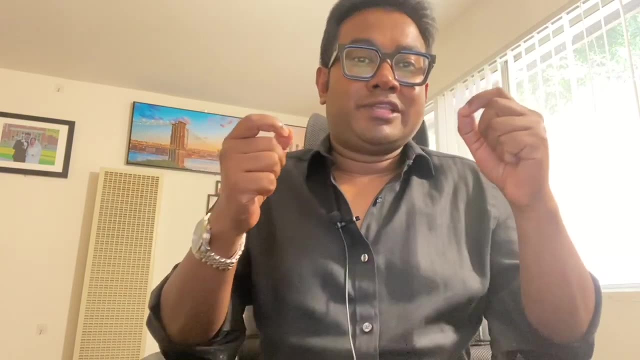 okay, which we know as an aeronautical engineer, so by default in any other country. if you say that, okay, i'm an aeronautical engineer, i'm an aerospace engineer, people essentially initially they will think that, okay, this guy is an airplane design engineer. okay, and if you want to become this, 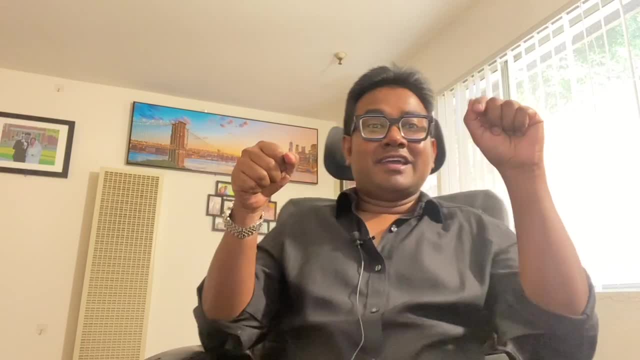 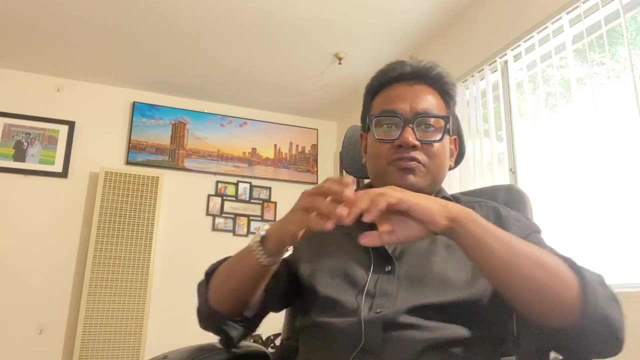 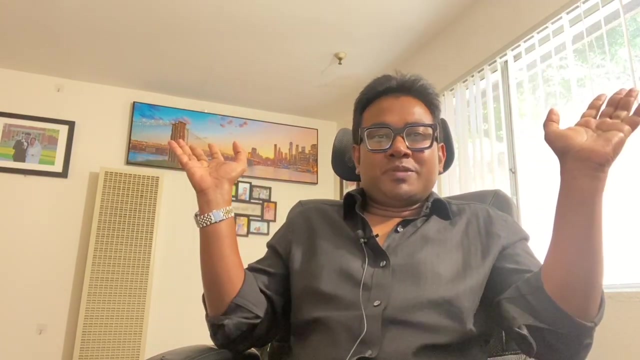 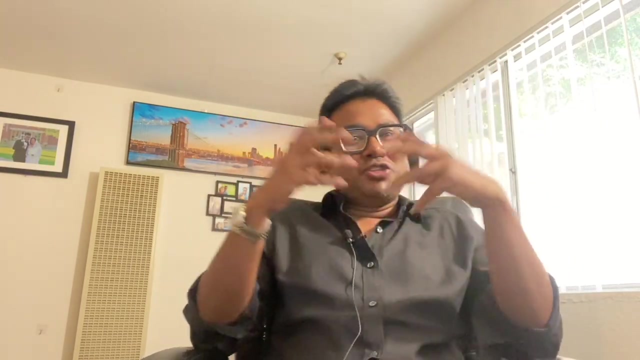 specialized person. you have to study aeronautical engineering and, more specifically in terms of bangladesh, you have to study aerospace. you have to take the aerospace track. But if you are someone who is not so much passionate about becoming an airplane design engineer, okay, I am happy with any types of job in Boeing, any types of job in any aerospace company. I have no specific choice that I want to become an airplane design engineer. then you can choose either aerospace or avionics.